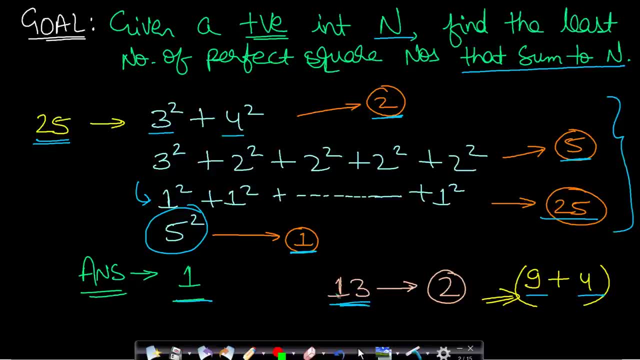 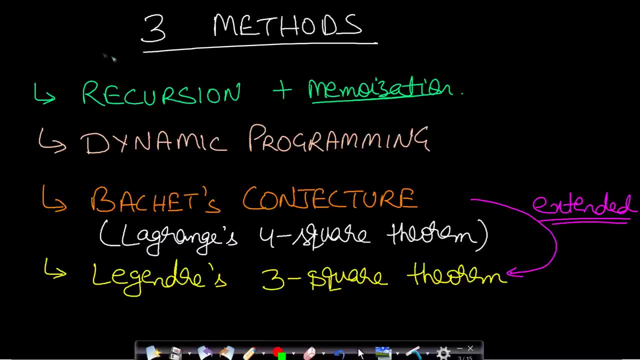 which will get better than this, since this 13 is not a perfect square in itself. okay, so in this case, we will simply return 2.. so i hope you got the problem statement. let us now look at the methods by using which we can solve this. so i will be showing you three solution methods. first one: 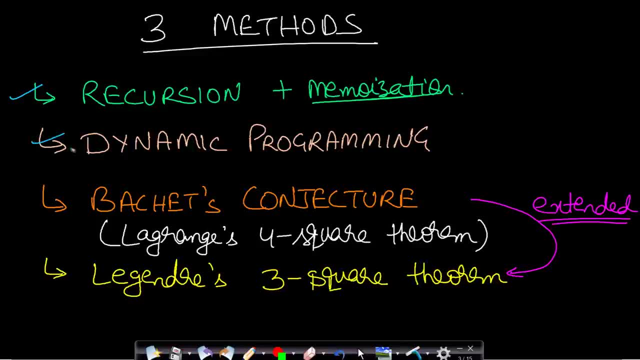 will be by using recursion plus memoization. second one will be by using dynamic programming tabulation method. and the third one will be by using lee gender's three square theorem, which is derived from the batchett's conjecture, also known as the lagrange's four square theorem. okay, so before. 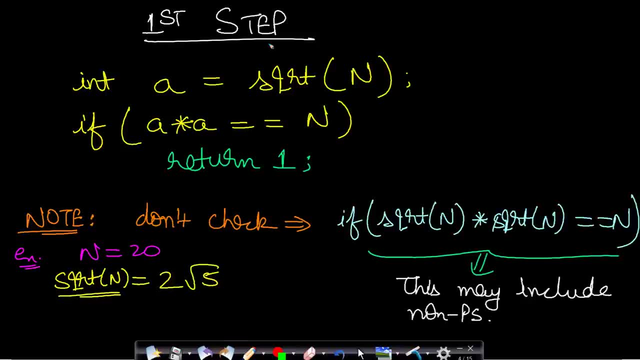 seeing any solution. let us move step by step. so the first step is: if you are given a number n, then you will check if it is a perfect square. if it is a perfect square, then you will simply return 1.. so in this case, square root of n should be stored in an integer value, and then only you. 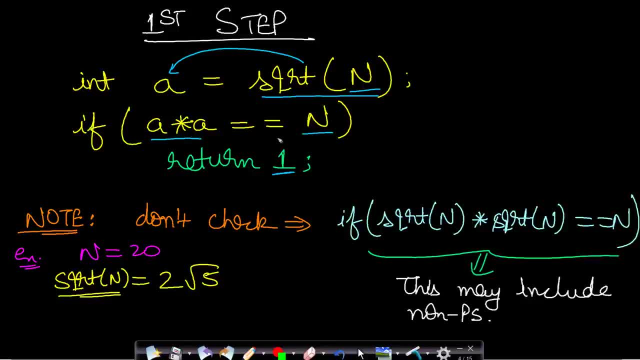 should compare a into a equals n, because if you do not do this and you do something like this, square root of n into square root of n should be equals to n, then this might include something like irrational numbers or some decimal numbers as well. you want that this a should be perfect square root of this n. okay, so for that reason you will, for 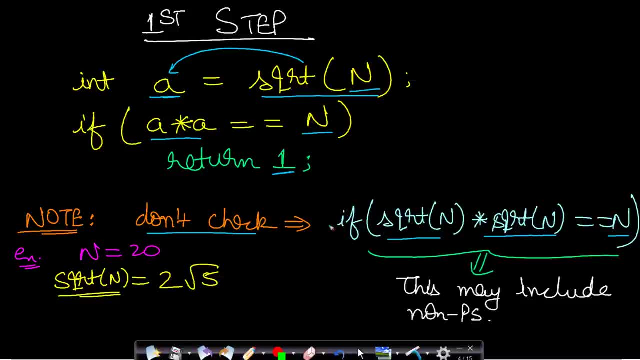 store it in an integer value, so this is not a good practice to use. okay, so let us say your n value is 20, then your square root of n will be 2 root 5. so if you use this method, then this one might give you the correct result that this one might produce. 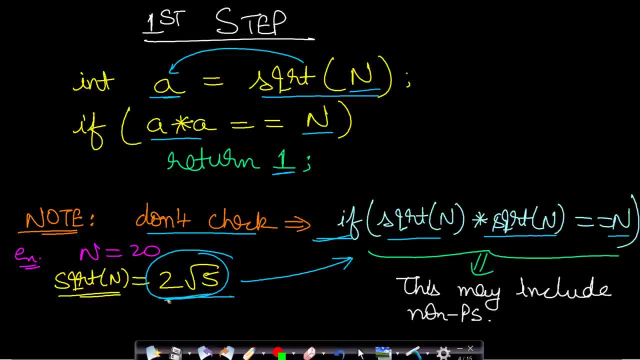 true, but you have to remember that this is a non-negative value and that is not a productive value. so, for example, if you use this method, then this one might give you the correct result, that this one might produce true, but this one might produce true, but then it will be false, because if you take an integer, then actually square root of n will be 2. 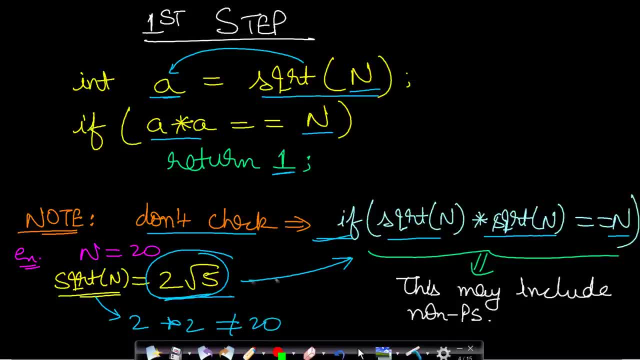 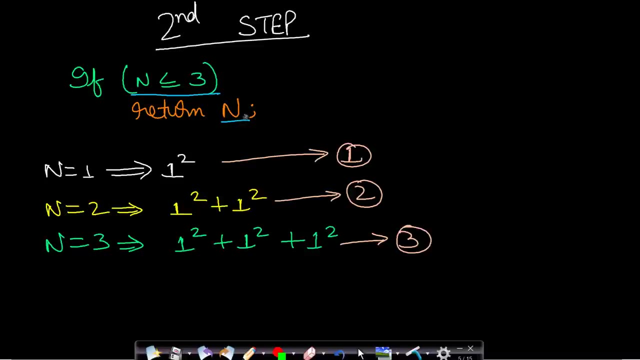 so 2 into 2 is not equals to 20, but if you use this formula, then this might give you true answer. okay, so better to use this method. now let us look at the next step. so the next step is: if your n value is less than equals to 3, then we will have to simply return n. and why is that? because if 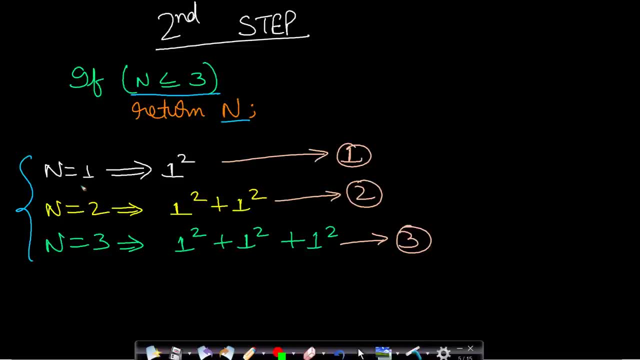 your n value is less than equals to 3, then there is only one possible split. like you can write n equals to 1 as sum of 1 square, you can write 1 n equals to 2 as sum of 1 square plus 1 square. 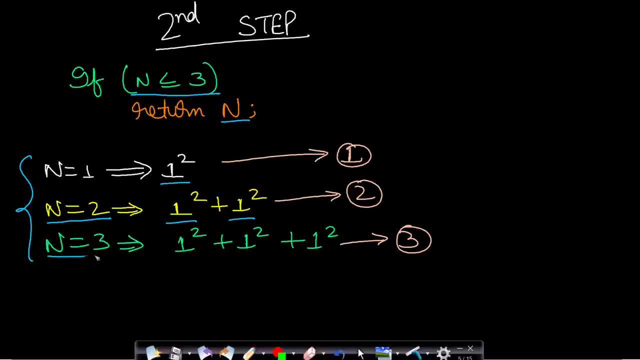 so these are the sum of two perfect squares. if you write n equals to 3, then this will be a sum of three perfect squares. okay, so for n equals to 1, 2, 3, you will simply return the n value, and if n value is equals to the 0, then simply you will have to return 0, since there is no possible. 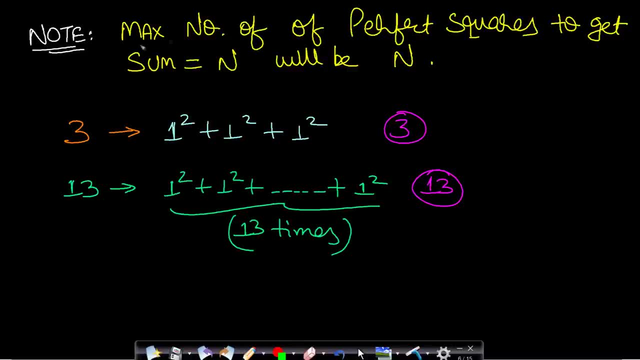 perfect square possible. okay, so the third step is: maximum number of perfect squares to get sum equals to n will be n. so, as i have shown you, like in the previous step, in this case this was the worst case scenario because, given a number n, let us say, if you are given the number. 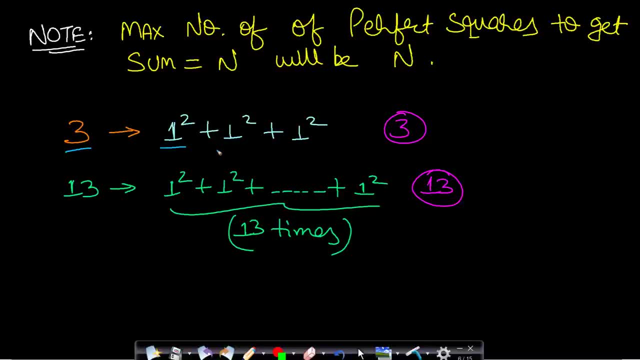 3, then it can always be split into chunks of one square. one square and one square. okay, so it will always be possible to break it into three parts. so, given a number, 13, it can be possible to break it into 13 parts, into chunks of one square, because one square is also a perfect. 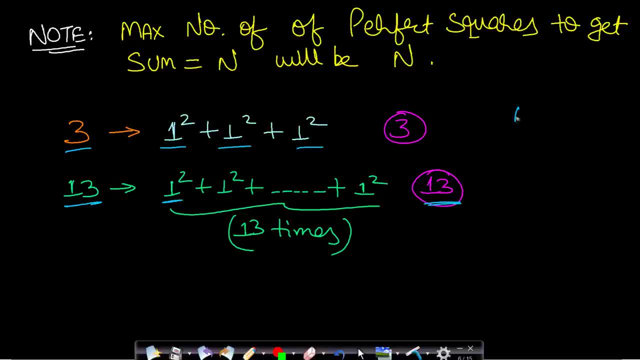 square, okay, so your answer will be 13. so, given a number, n, in worst case we can get this n by n divisions of one square each. therefore, for n, the worst case answer will be n. so we need to find the minimum answer. okay, and it can go maximum to n. so this is one important point to note. now, given n, 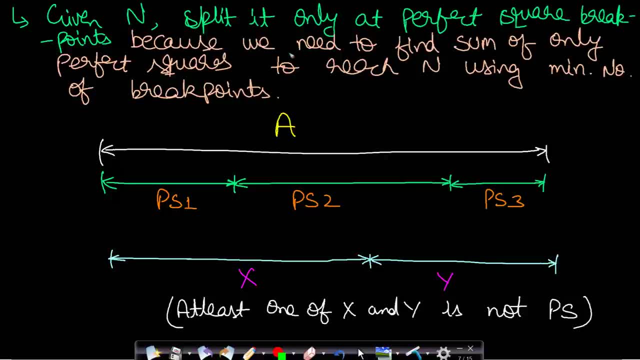 split it only at the perfect square breakpoints, because we need to find the sum of only the perfect squares to reach n using the minimum number of breakpoints. so let us say your number given is a okay, so you cannot simply break at any point, like if you are considering this a for. 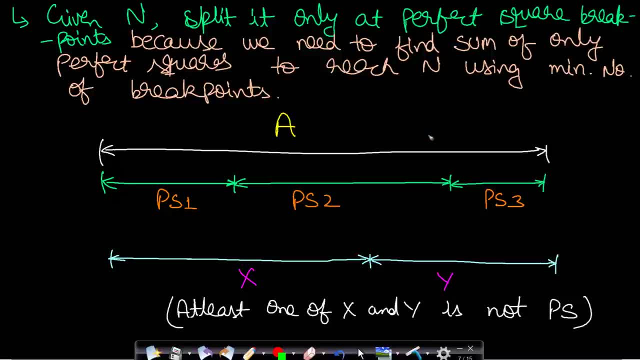 breaking it into perfect square sums, then what will be the value like? wherever you break, it should come out to be a perfect square. okay, so let us say i will move from the right hand side. let us say this is a and this is 0.0. okay, now where should i break? let us say i break at this point. then whatever the 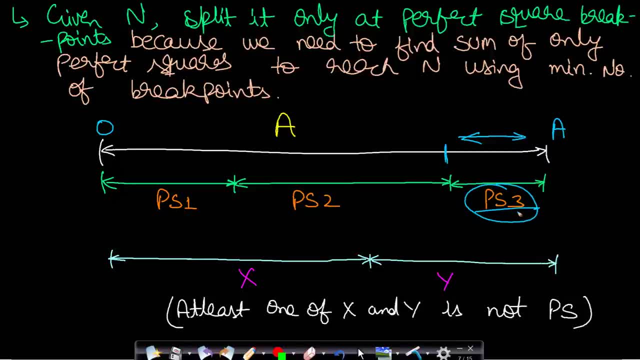 value is like this ps3, this one should be a perfect square, otherwise i cannot put a break point here, because the question says that we need to get this sum a by using the sum of perfect squares. so we cannot just break at any point. now let us say the next point where we can break is: 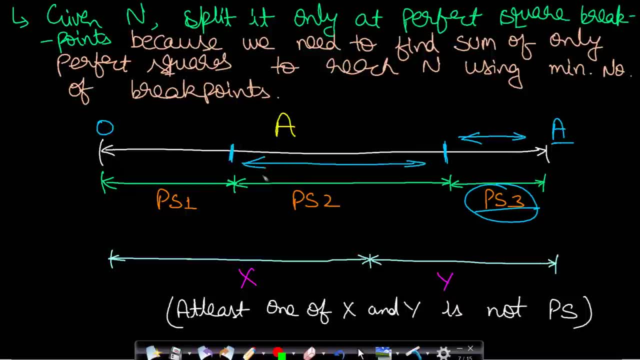 this point, then this value as well should be a perfect square. so this ps2 should also be a perfect square. and also, if you break like this, then ps1 should also be a perfect square. only then you can add these three values and get this value a okay. so this number line is basically: 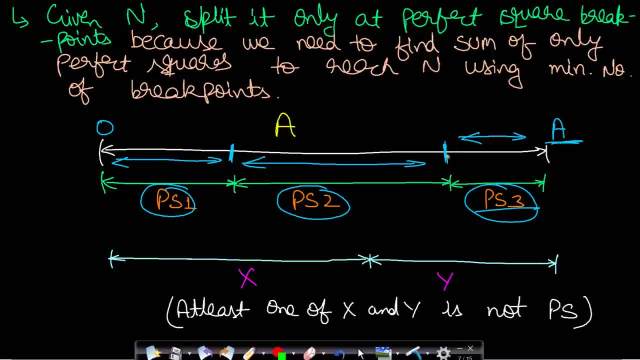 starting from zero, because we are dealing only with the positive numbers. so in the second example you can see that you cannot just break at any point. so this was our first break. point b1 and this is our second example, and we can see that we cannot just break at any point. so this is our. 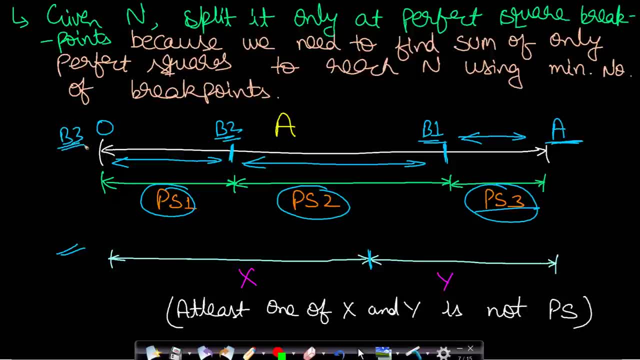 second breakpoint: b2. this is our third breakpoint. let's say it's b3, then in this case you can see that this point is lying between b1 and b2, so we cannot do a break at this point. since the last point is also a, so at least one of x and y is not a perfect square, then we cannot do a breakpoint at. 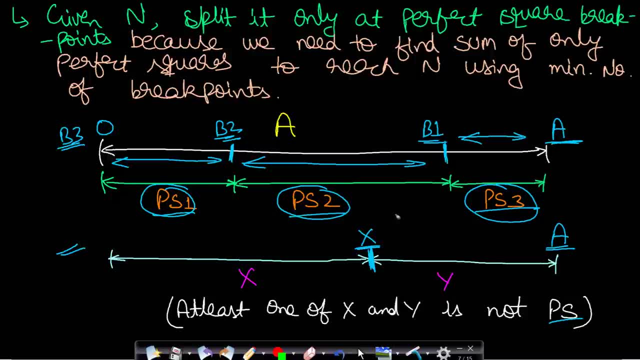 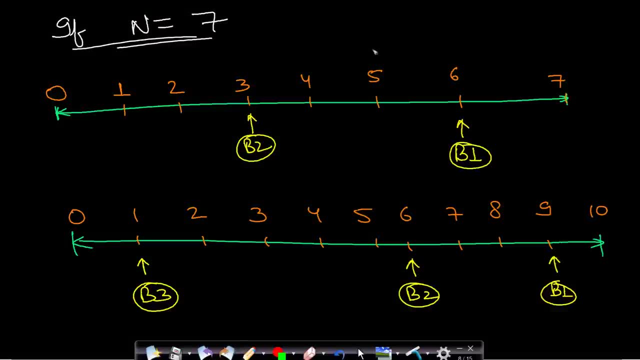 this point, because all the parts, that is, all the chunks, should be a perfect square. this is the main constraint of our problem statement. okay, so let us say your n value is equals to 7, so this is the number line which i have drawn. now, where can you put the breakpoints? the first breakpoint can be: 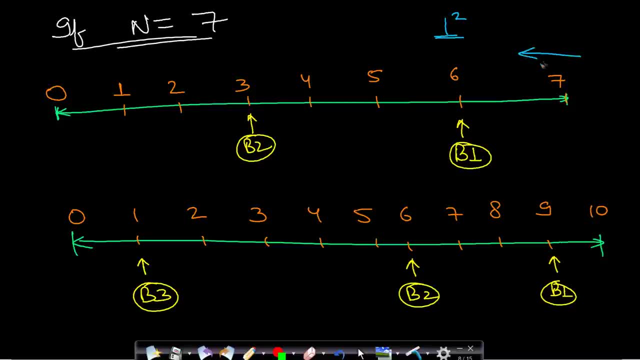 at a difference of one square. so let us say we are moving from right to left, then at one square you can put a breakpoint. so this is one square and hence you can put a breakpoint here. okay now, if you consider this 7 again as your starting point and if you want to find the next breakpoint, 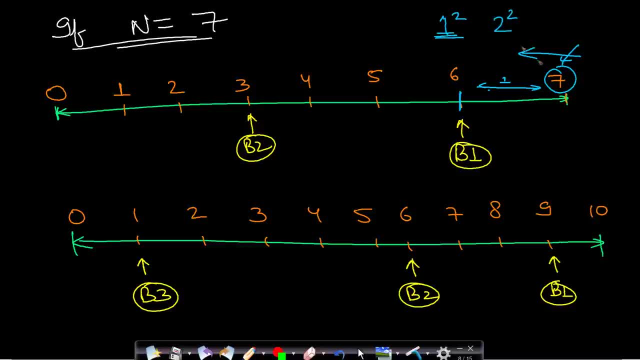 you can put a breakpoint here. and if you want to find the next breakpoint, you can put a breakpoint here. and if you want to find the next breakpoint, you can put a breakpoint. then that can be a two square. so what is the two square difference point? it is three. 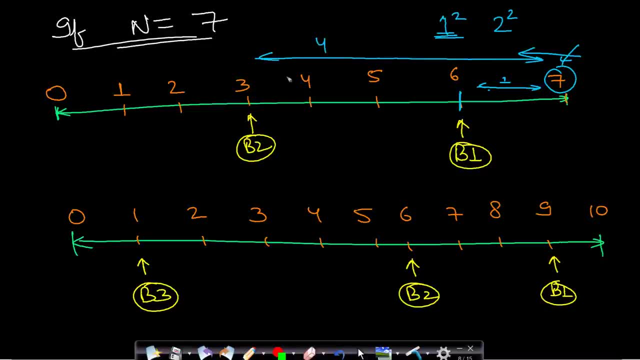 because this difference is two square, which is four. okay, so the next break point will be at three. and what will be the next break point? if you consider this seven as your starting point, this will be three square. so three square will be nine, but nine will be out of bounds. 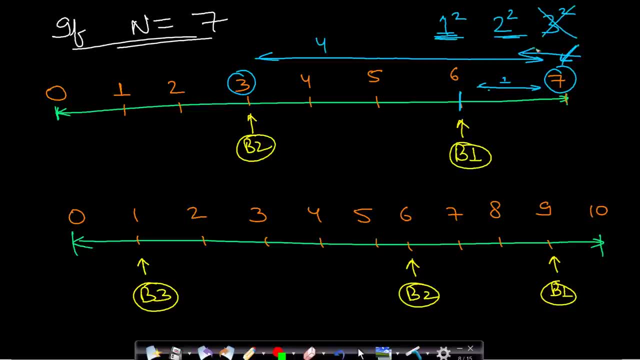 so you cannot do this break point. so there are only two break points if you are starting at seven. but let's say you used this one square break point and went to six and then from here you can again do a one square break point or a two square break point, choosing this five. 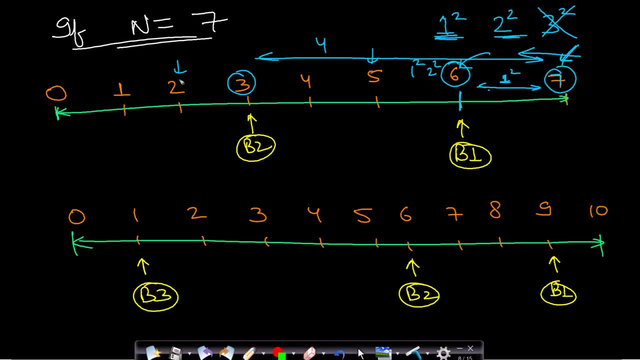 otherwise this two. okay, so this is a recursive process actually. so if you see the second example in this case as well, if you consider this 10 as your starting point, then you can put a break point at one square difference, which will be at nine, at two square difference, which will be at six. 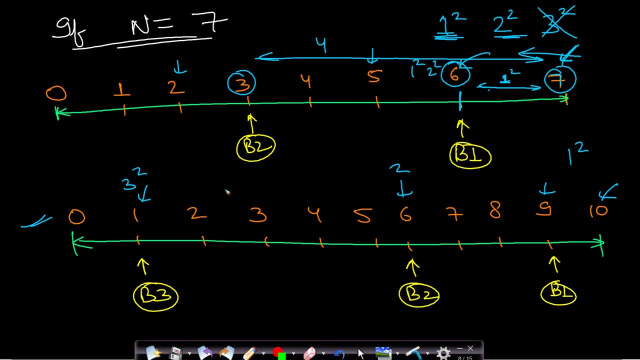 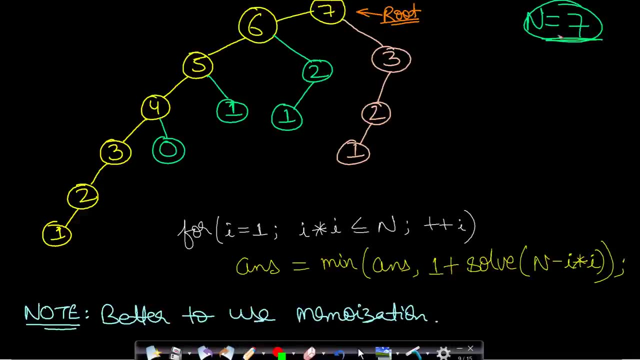 and at three square difference, which will be at one. okay, so i think you understood this breakpoint approach. now let us look at how do we solve it. by using recursion. so let us assume that our n value is equal to 7.. so this is the recursion. 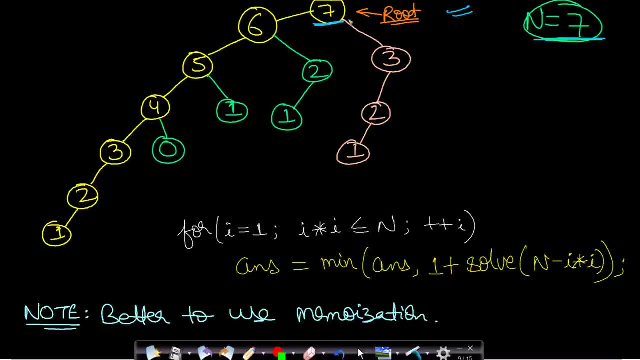 tree actually, which will be drawn. so this is our root, which is 7.. so how do we break this point? actually, if n is equals to 7, then we will start with the minimum possible breakpoint size, which will be one square. so if you break it into one square, then this 7 will be called with the value. 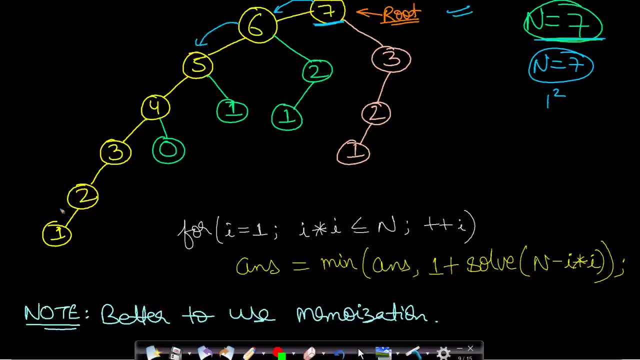 6. again, this six will be a 6. then the break point will be equal to 7. so if you work this out, then this will be equal to one square. then this seven will be called with the value 6. again, this six will be broken into 5 and so on. this will be broken to size 1, and let us say your base case. 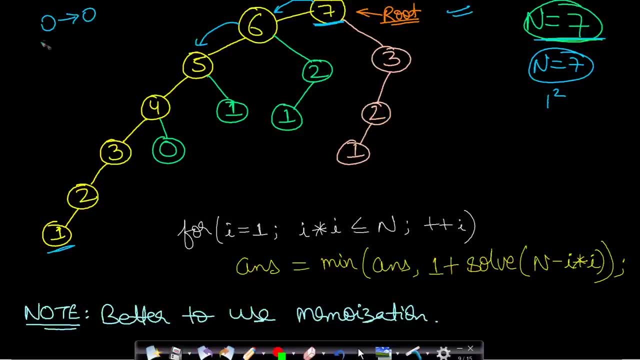 is that for 0, you will return 0, as i have already explained you. for 1, you will return 1. actually, you can also do like this: for n less than equals to 3, you will simply return n. okay, so it all depends on you. how do how you do it. so in this case, i will assume that i have used only 0 and 1 as our. 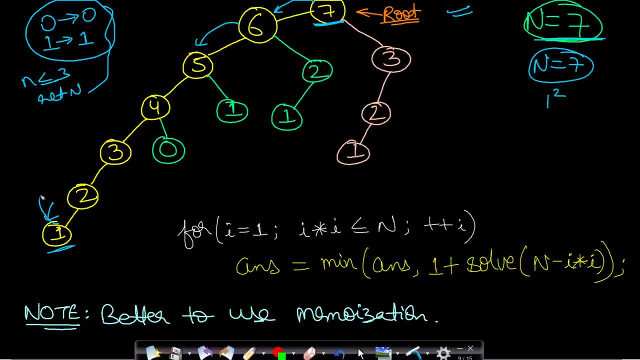 base case. so as soon as we reach this 1, then this will return 1 here. okay, and then this will try for the second breakpoint. but from 2 you cannot have a breakpoint of size 2 square, so there will be no right call, this will just be a single call. so this will be returning a value 2, which will be 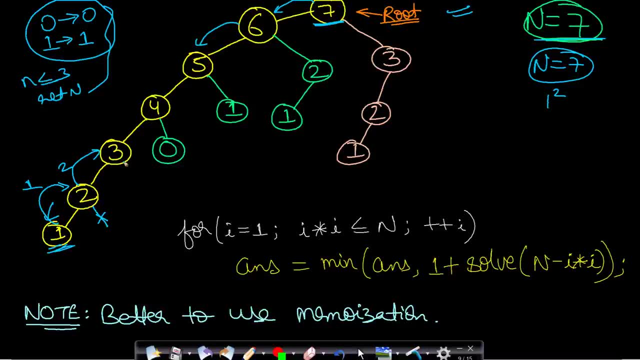 1 plus 1. now this 3 can also not have more breakpoints, because more breakpoints will make it go out of bounds. so this will return a value 3, which will be 1 plus 2, because we have put the breakpoint at 3, we have put the breakpoint at 2 and we have also put a breakpoint at 1. so this 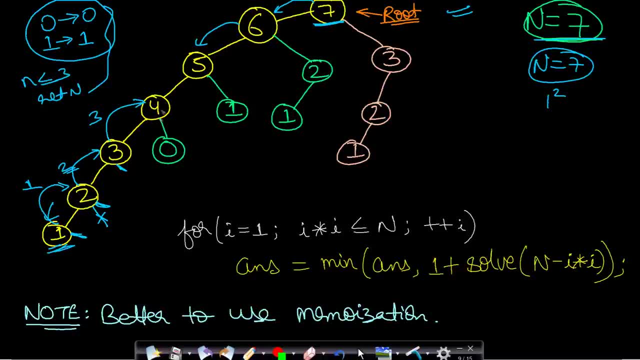 is nothing but the count of breakpoints actually. so at 4 you can have the second breakpoint, which will be 2 square, and the value will come out to be 0 here. so for 0, we know that answer will be 0, so this will be returning 0. 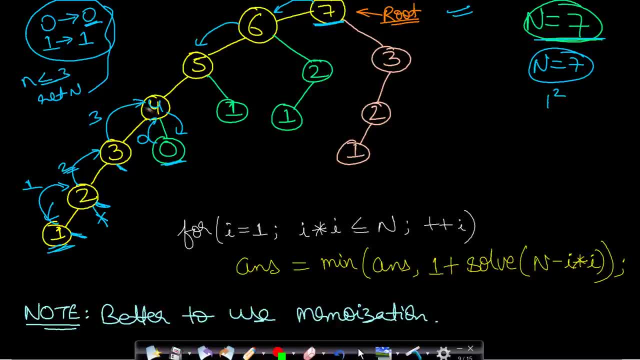 and so this will be returning the minimum of this: 1 plus 3 comma, 0 plus 1. okay, so this 4 is actually a perfect square. therefore, we will simply return 1. okay, so for this 5, it got from the left call value 1. it will make the breakpoint of size 2 square and the value will come out to be 0 here. 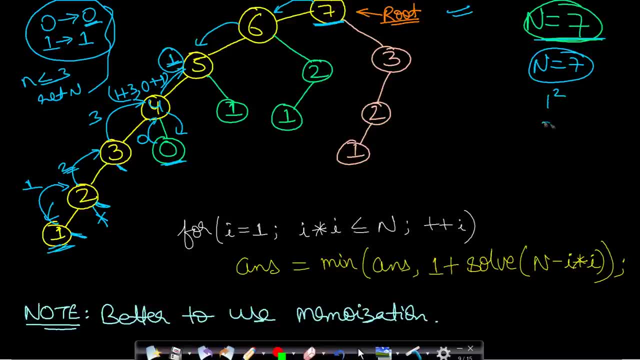 so for this 5, it got from the right call. it will do the next split. so the next split will be at 2 square difference, so it will be at 1. so 1 is a base case. it will be returning the value. so, similarly, this entire tree will be traversed and you will get your optimal answer at the root. you will take. 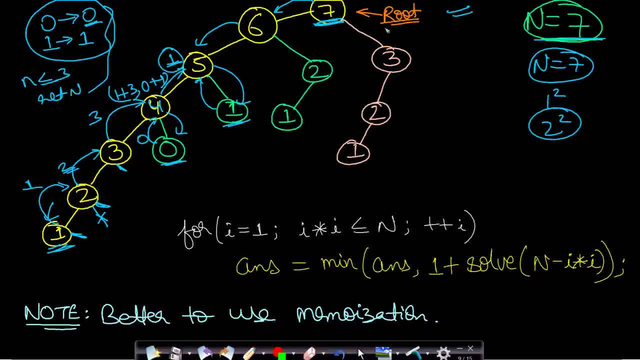 the minimum of all the calls. okay, so how do you implement this? actually, these are the two lines which is very helpful for implementing this approach. so this for loop is actually creating the breakpoints. so your breakpoint can start from the left call and the next call can start from the. 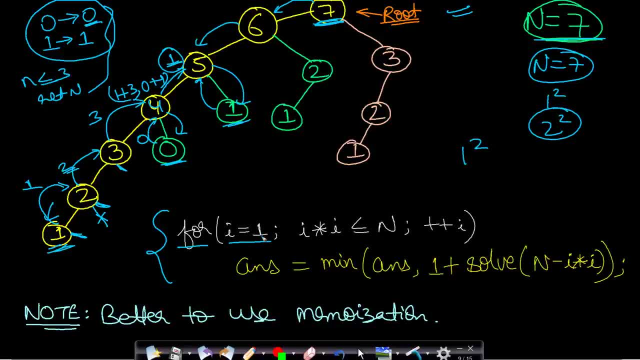 right form for loop. however, if you separate the number from this breakpoint, you will say: in fact, the breakpoint is moving higher, which is a result of not anticipated by the observer. and if your useful comment is not k or when you launch your call, then the second技� śr desc doesn't come out necessarily. the second falloff, isential in, means. i will say: if we create value 1, it will stay inside, go out and okay again. in plus comes H, alpha to the limit n. now you will select the creores qua. i equals to n in balance, that is should than equals to n, okay, and you will increment i by value one. now, when you make the recursion called, then actually you will be decrementing the. 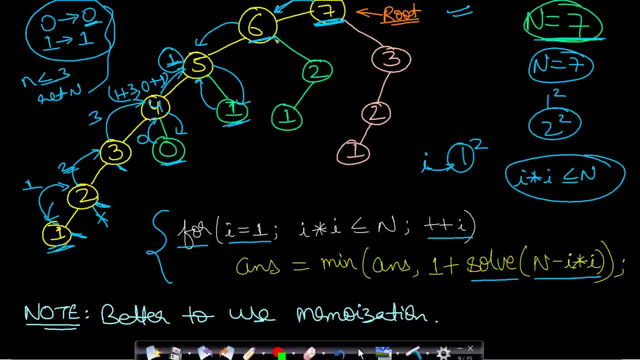 taking break of 1. okay, so you reached this 6. and similarly, you will make a break of 1 and you will reach at 5. otherwise, if you do a break point 2, then 4 will be reduced from it and it will make a call to 3. okay, so these are basically defining the break points n minus i into i will give you. 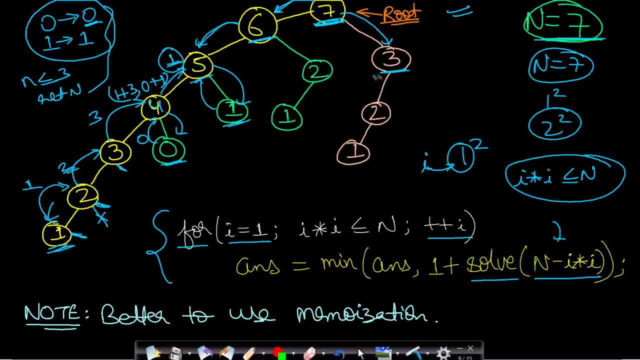 the next break point. so if you solve this smaller problem for this 3, then you can solve this bigger problem. okay, and in this case as well, you can see that there are many repeating sub problems. this 3 here and this 3 here is a repeating sub problem. this 2 here. this 2 here is a repeating 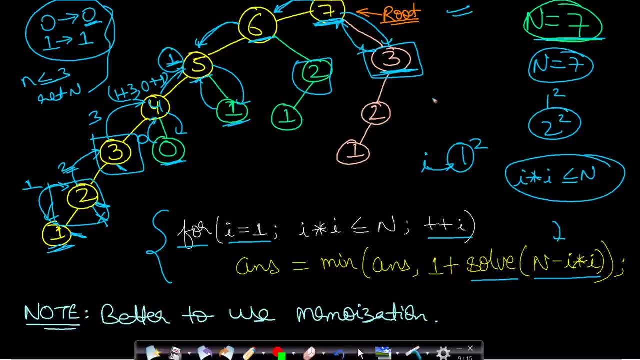 sub problem and there will be many other repeating sub problems as well. okay, so there are repeating sub problems and also, if you solve the smaller sub problems, then this will lead to a solution for the bigger sub problems. therefore, there is optimal substructure as well. therefore, we can. 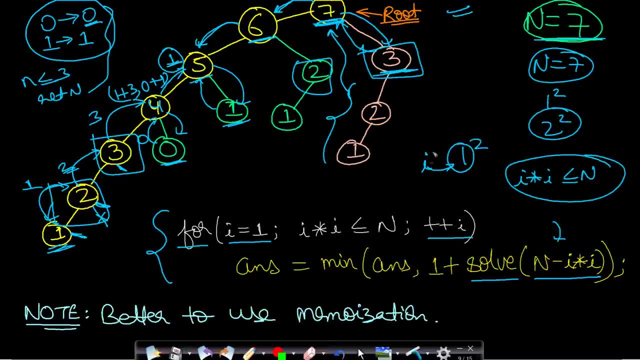 solve this problem by using dynamic programming you, so you can use memoization. okay, memoization will do like: if you come to a value and if it is not calculated, then it will be calculated and stored in your table. and once you have calculated and stored in your table, and the next time when you encounter this value, then you will simply look. 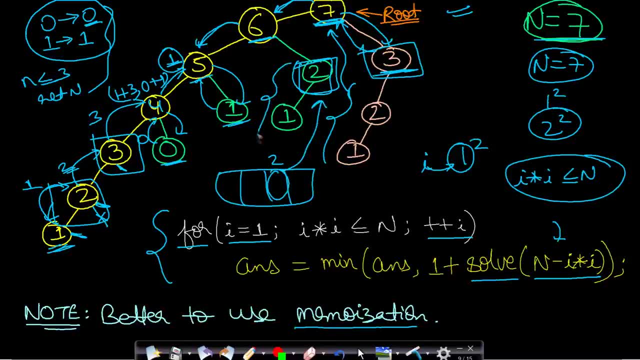 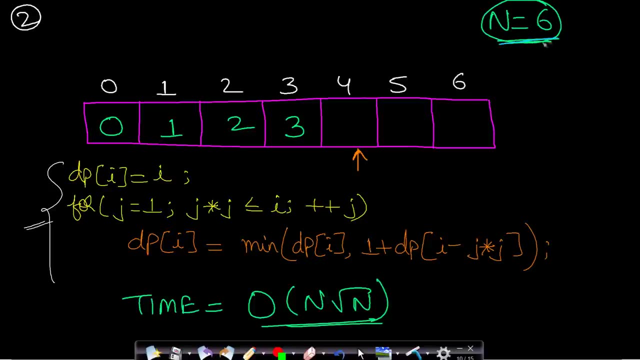 this table and return the value so that no further processing is done. so this lookup table will help in removing all the unnecessary recursion calls. so it is better to solve this by using memoization. now we can also solve this by using dp tabulation method. so let us say our n. 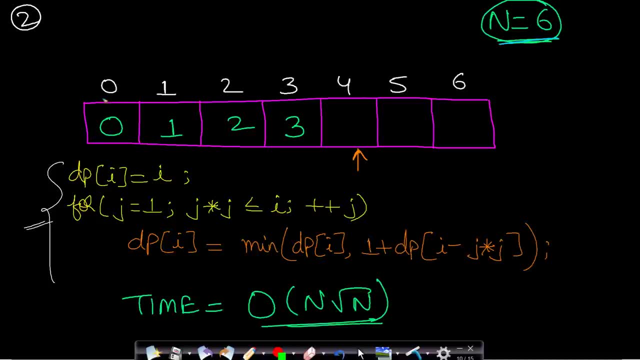 values equals to 6. so in this case, i will write 0, 1, 2, 3, with value 0, 1, 2, 3. as i've already explained, these are the base cases, so i will start with a value 4. okay, so basically what i will do is i will 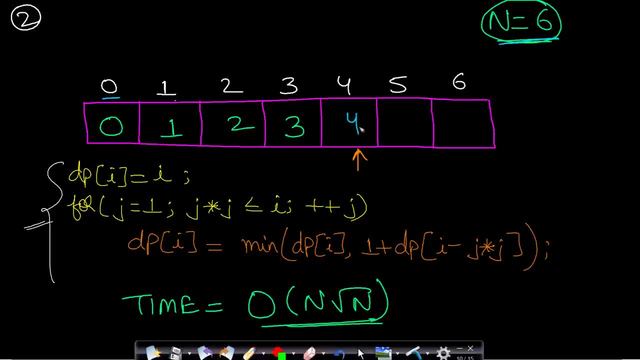 assign this value 4 with 4 initially because in the worst case, any number i can be divided into chunks of 1 square, as i've already explained. so i will write 0, 1, 2, 3 with value 0, 1, 2, 3, as i've already explained. 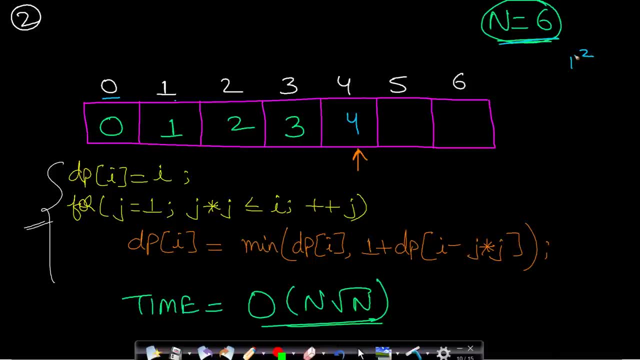 you. so if you divide a number in chunks of 1 square, then how many chunks will be formed? there will be n chunks. so for this n value 4, the answer will be 4 initially, because this is the maximum possible answer. now you want to minimize it. so how do we minimize it actually? so in this case, 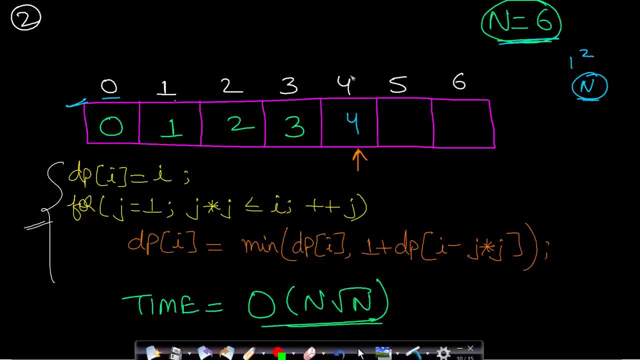 we have already filled from 0 to 3 and now we want to make optimal result for this 4, so we will start with the breakpoints. so we will start with the breakpoint 1. so 1 will be making a breakpoint of size one square, so we will go to the previous value, one square. and 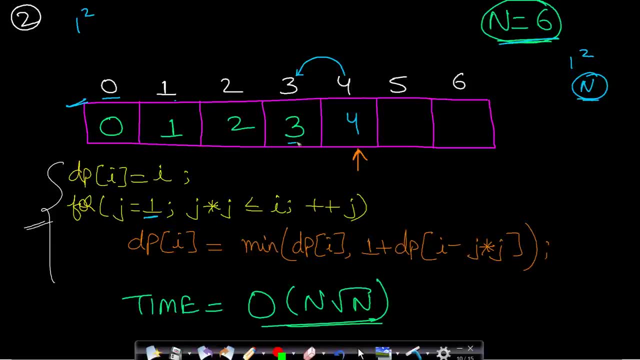 what is the value here? for getting three, you need three chunks. okay. so for getting four, how many chunks do you require? actually, you made one split in order to reach this three, so the number of chunks required to make four will be one plus three, which will be equals to four. but then 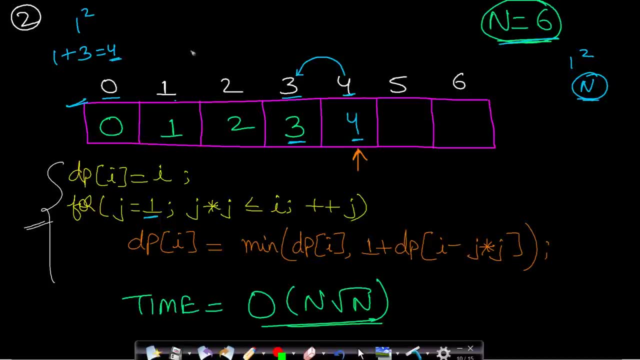 you will take the minimum of whatever is stored here plus whatever you found in this call. so this call, you found four and four is already stored here. so nothing will be done now you will try for the next breakpoint. so what will be the next breakpoint size? the breakpoint size will be: 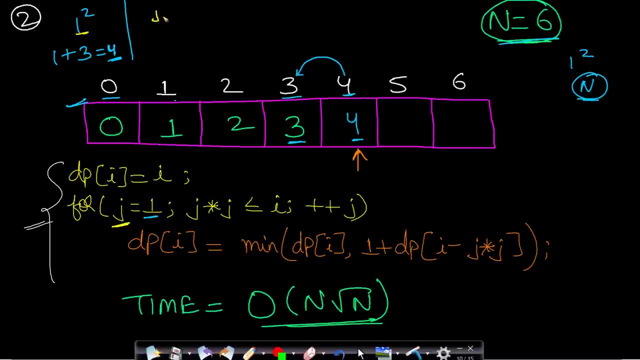 defined by this j value. so j value will be two, so breakpoint will be two square. so if you go to two square, then you will simply reach this value zero. so you have made one split and you reach to value zero and answer here is zero. so what will be the number of square sums in order to get this four? 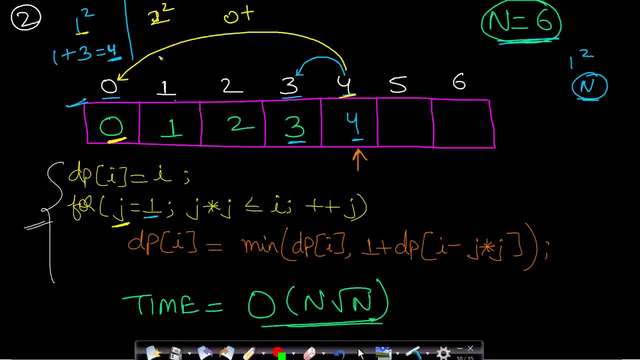 it will be this zero plus the number of splits you made. now you are making just a single split, therefore it will be one. so you will take minimum of 1 comma 4, so this will come out to be 1, and now you cannot make further breaks because it will go out of bounds. so you will now move on to the next. 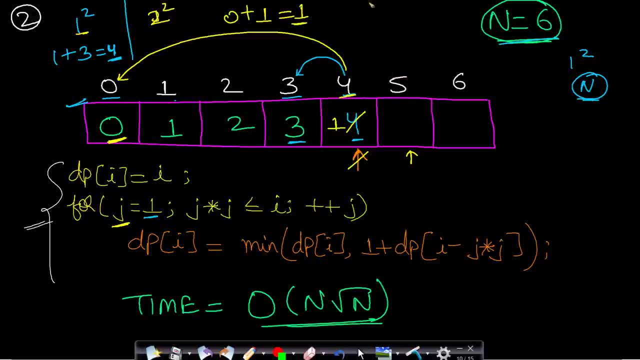 step. so for this value, n equals to 5. similarly, you will repeat the process. the j value will start from one. okay, so this is j value loop. so in this case as well, the first split will be the number of plus. it will be zero, so you can now go out of bounds. and also you will have the number of square. 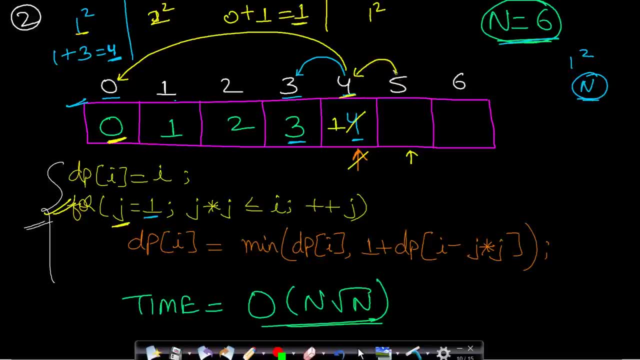 be at a difference of one square, so you will reach this four. so you can see that you can form this four by just using a single split. okay, that is basically by making no split at all. so in this case, in order to form five, how many chunks do you require? you will require number of chunks in order. 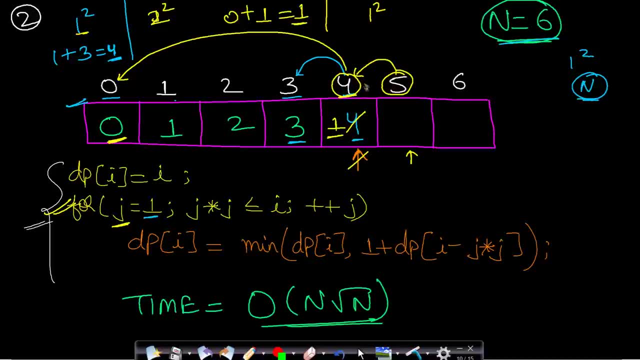 to make four plus one, because you are making a split at four. so it will be one plus one, which will be two, but initially you will fill it by five because this is the maximum number of chunks which you can use to form this number. so now you got a number two, so you will update this value to: 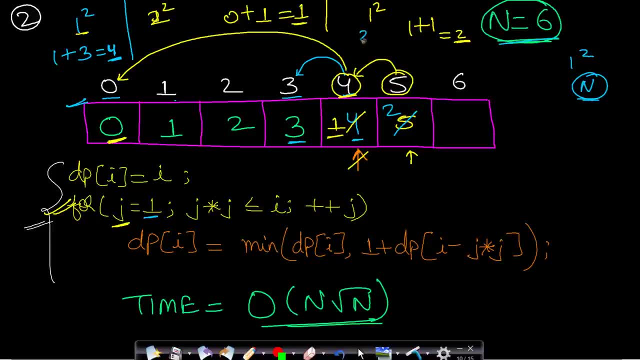 minimum value, which is two. now you will simply do the second split at two square. so if you do at two square, you will reach this one. so what is the value at one? it is one, so one plus one will be two and it is already two. so you will not update it and you cannot make further splits. 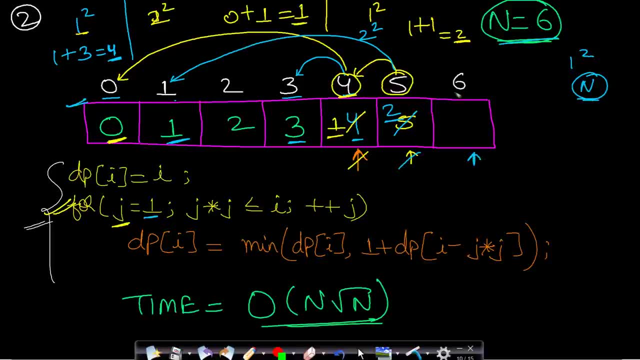 because it will go out of bounds. so now you will do: for n is equals to six, so for six you will do a one square. split at five, it is two, so here it will come out to be three, but it will initially be filled with six, which is the. 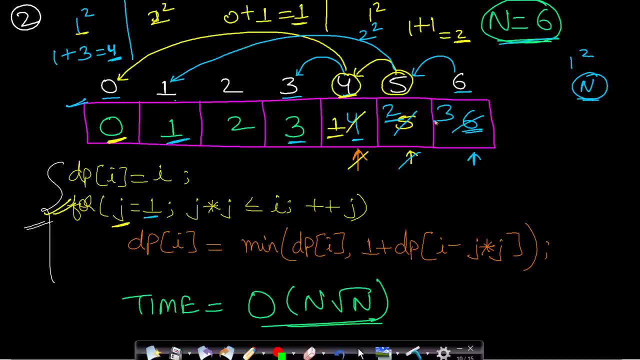 maximum number of chunks required, and now you got three, so you will update it with three, since this is smaller, now you will make a two square split. it will be at two. two's value is here two, so two plus one will be three. it is already three. now three square split is not possible, so you will 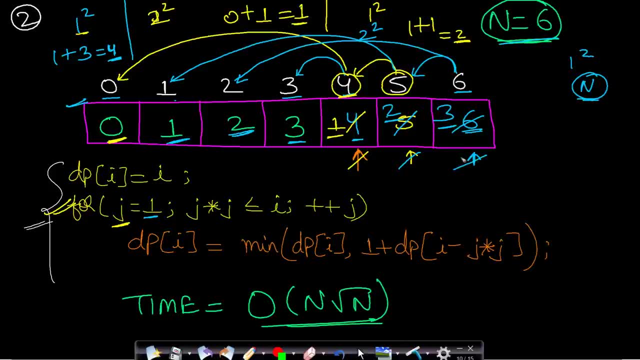 not do anything now. finally, after processing each and every value, you will return dp table, dp at n. okay, so this is our dp table. so dp at n is equals to 3, so in this case, the answer will be 3. okay, so what will be the time complexity? actually, we are covering all the n values. 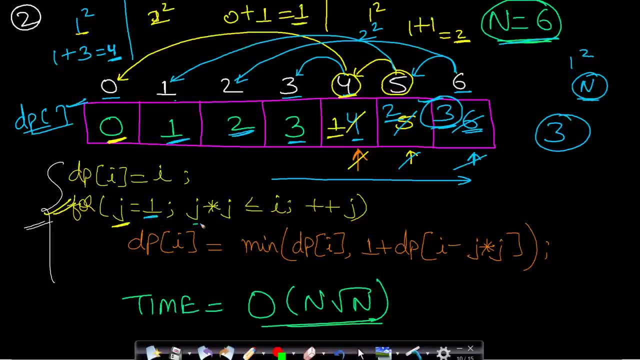 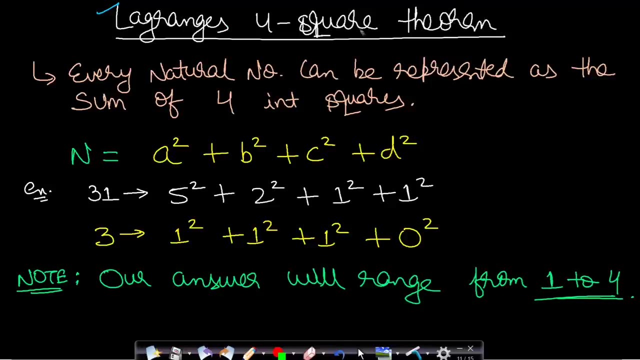 and for each value we are making split from 1 to j into j less than equals to i, which is nothing but square root of n. okay, so the total time complexity will be n square root of n. so let us now look at the next method. so the next method is based on lagrange's four square theorem. 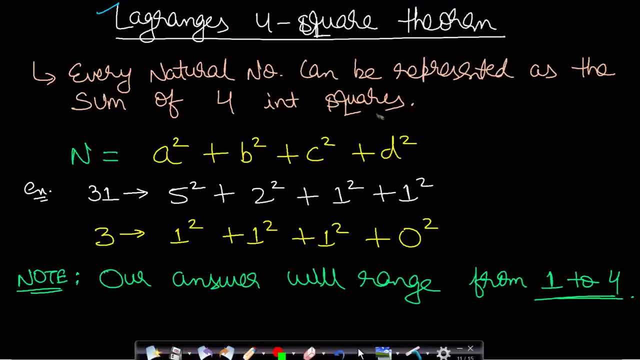 every natural number can be represented as the sum of four integer squares. so if your number is, let us say, n, then it can be represented as a square plus b square plus c square plus d square. so, let us say, if your number is 31, then it can be represented as 5 square plus 2 square plus 1. 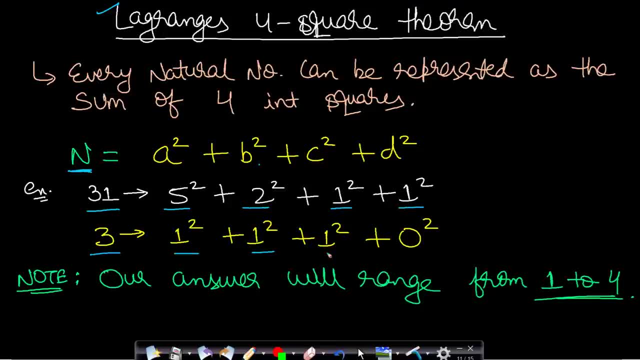 square plus 1 square and 3 can be represented as 1 square, 1 square, 1 square and 0 square. so you can see that for our problem, our answer will range from value 1 to 4. this is for sure using this lagrange's. 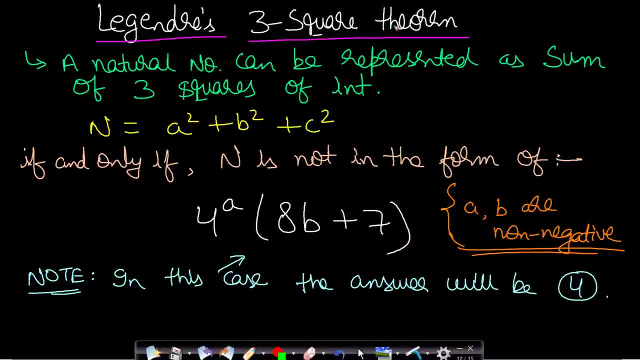 four square theorem. okay now, legendre's three square theorem is actually derived from lagrange's four square theorem, and it says that a natural number can be represented as sum of three squares of integer. so if your number is n, then it can be represented as a square plus b? square plus c. 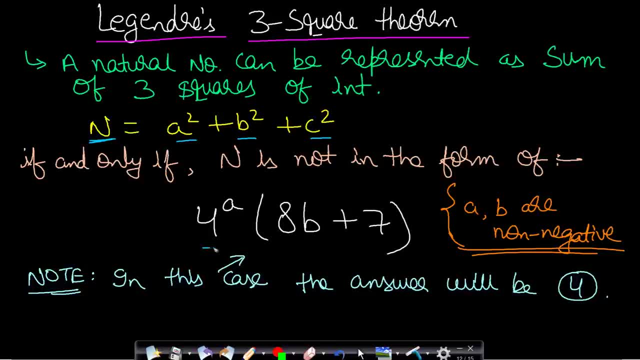 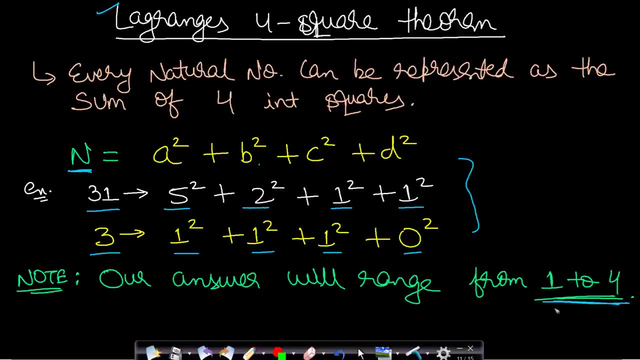 square if, and only if, n is not in the form of four, to the power a multiplied by eight, b plus seven, where a and b are non-negative integers. so in this case the answer will come out to be four. okay, so we have already seen in the lagrange's four square theorem that our answer will range from one to four. 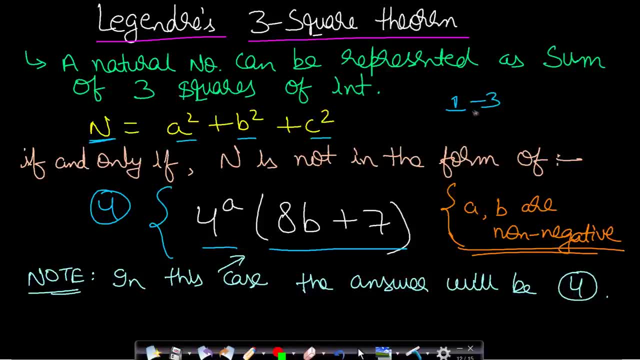 and in this case it says that it will range from one to three. but then if your number is of the form of this, then you can represent it by using sum of four squares. okay, so if your number is in this form, then you will simply return four. now let us see how do we use this legendre's three square. 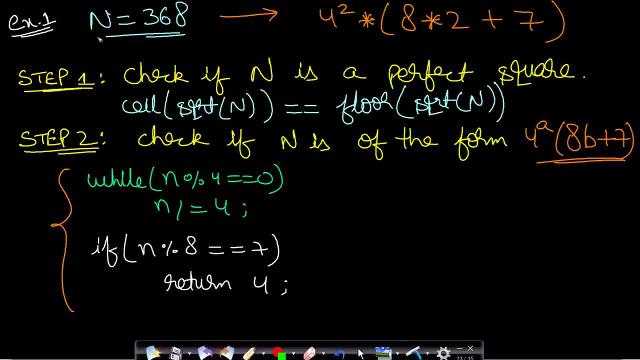 theorem in order to solve our problem. so let us assume that if your n value is equals to 368, now do? i have already explained you that first you will check if it is a perfect square. if it is a perfect square, then simply you will return one. so if c love square root of n is equals to floor of. 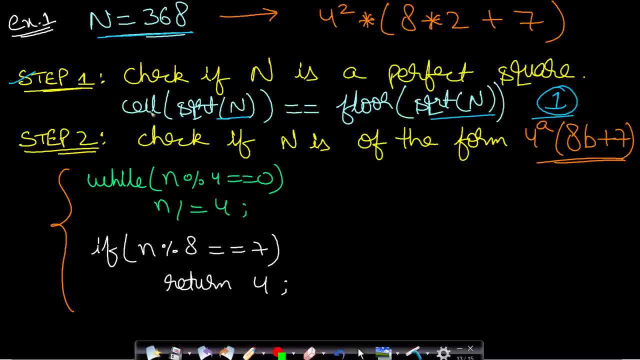 square root of n, then you will return one. okay, so if it is not a perfect square, then the case for this one value is gone now. okay, now we will check for case four, that is, if your answer can be four. now check if the number is of the form of four to the power a into eight, b plus seven. 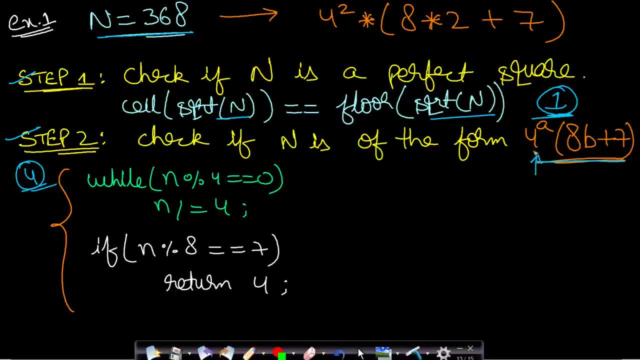 how do you check this? actually, you will keep dividing the number by four. so unless and until the number is not divisible by four, you will not stop. okay, you will keep dividing the number by four. so when you come out of this, then your number can be in the form of eight b plus seven. if your 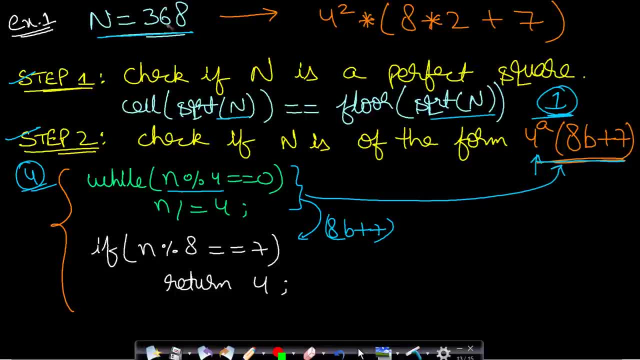 number was initially in the form of this one. okay, so if you take this 368, then actually your result here, before entering this, if statement will be eight into two plus seven, which will be nothing. okay, so now you will check if n mod eight is equals to seven. if it is equals to seven, then 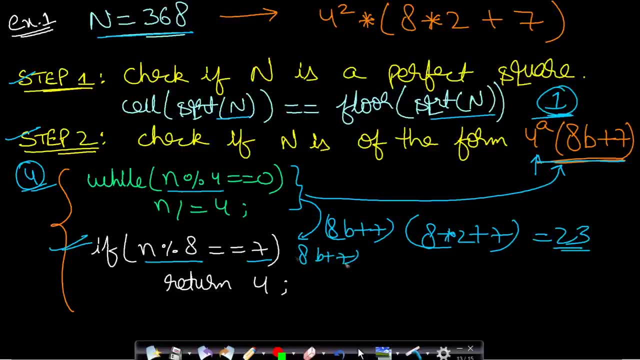 this indicates that number is of the form of eight b plus seven. so in this case, if you take mod eight for this value 23, then it will come out to be seven. so simply return a value four, because this number, 368, can be represented by using sum of four perfect squares. okay, so this: 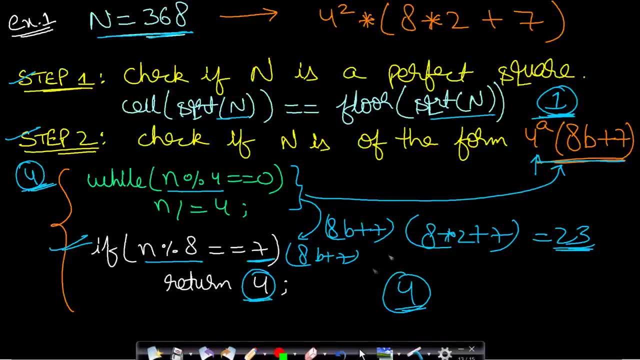 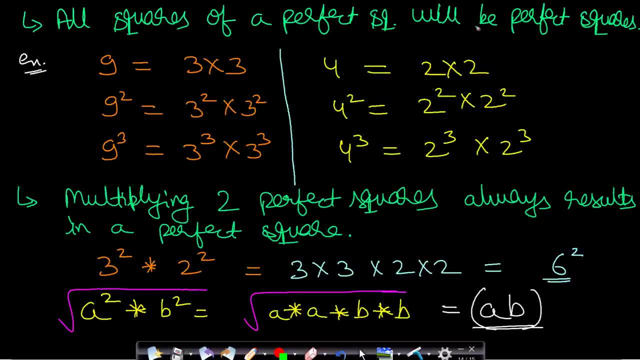 is according to lee gender's theorem. so we have only covered two cases only for value one and four and three now. so i will show you more cases as well. so all squares of a perfect square will be perfect square. so this is very simple to understand, i think. now the second point is that multiplying 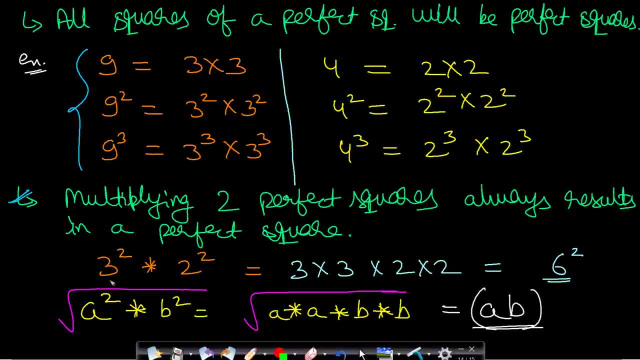 two perfect squares always results in a perfect square. so if you multiply three square into two square, then this will be three into three, into two into two, so this will be nothing but six square. now, if you take a general form like a square into b square and you take square root of this, 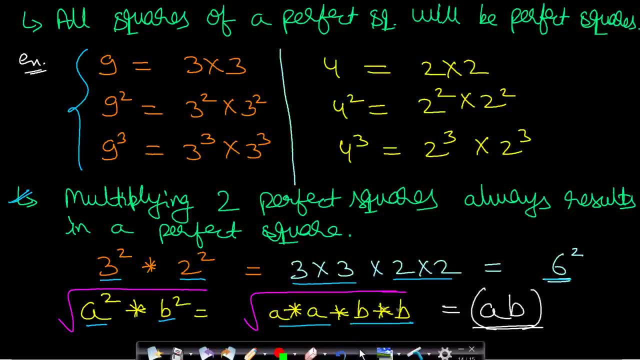 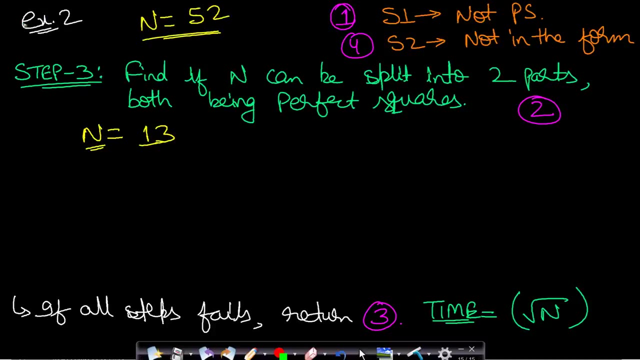 then this can be represented as b square, because they are in pairs. and now for the square root. actually, you will dissolve this pair into one, so this will be nothing but a into b. so multiplying two perfect square will always result in a perfect square. so this is the proof for this. okay, now let us look at this example. 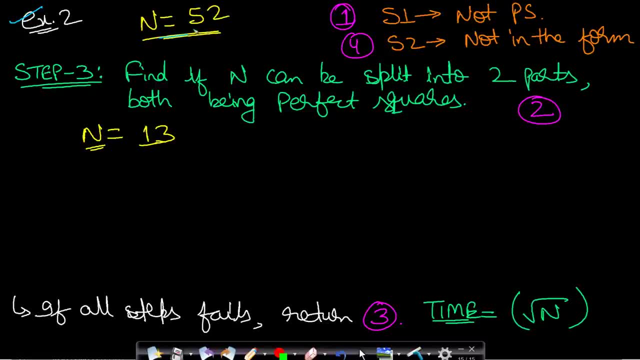 two. here n value is equals to 52. now this 52 will pass through this step one and step two. so when this passes through step two, then the n value will be reduced to 13, because we were basically dividing the number by four, unless and until it is not divisible by four. so the result: 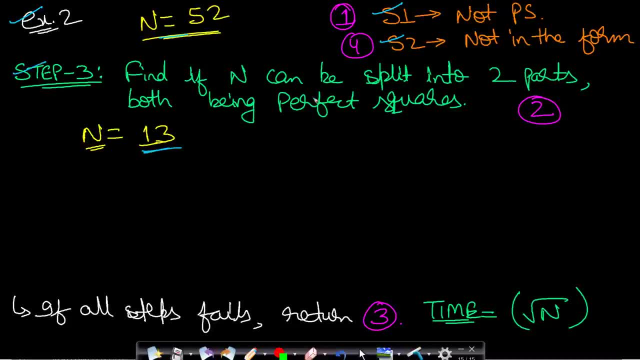 will be 13.. so in step three, actually, what we will do is we will check for a break point. that is, we will check for a point where, if we put a break point, then basically the left hand side will be a perfect square, the right hand side will be a perfect square, and on adding this, we will simply 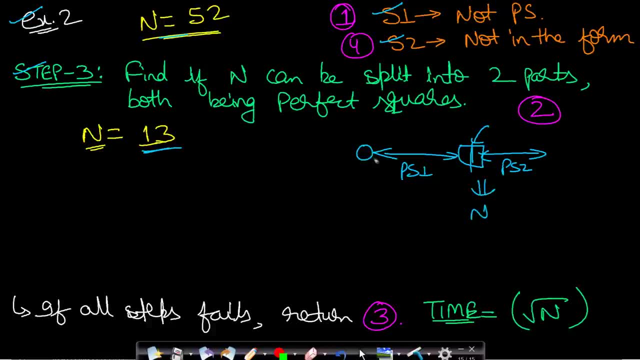 get our number n, so this left part should start from zero and this should end at value n. only then you this can be valid. so we want to find just a single break point. now, how do we find it actually? you can take this reduced value, it will also work. and you can also take this initial value, it will also work. 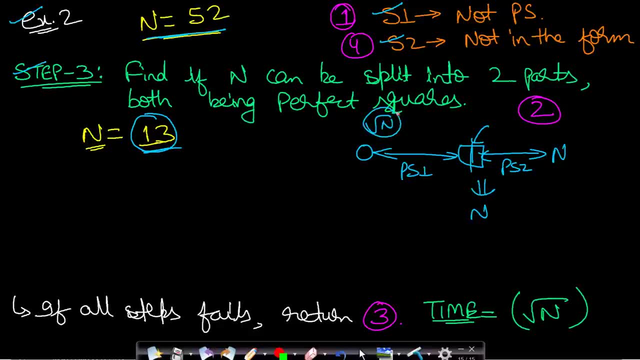 so this you can check it in square root of n time. okay, so how do we find this break point? actually, if you are having a number line, and let us say it is starting from zero and this is your value n, then you will put a break point somewhere and then you will see that this will be. 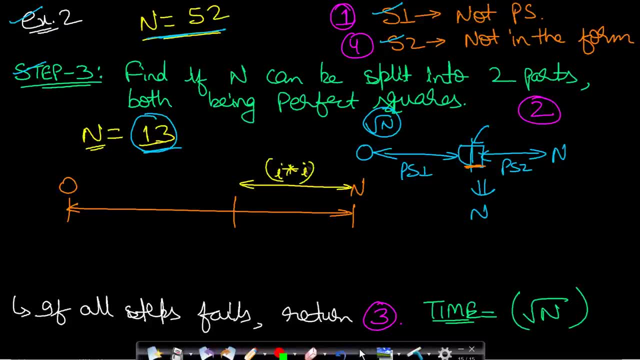 i into i. so you will run a loop and you will put the break points, as i have already explained you, in dynamic programming and recursion. okay, so when you are making a break point, then you are sure that this part is a perfect square. okay, now you want to verify if this part is also a perfect square. 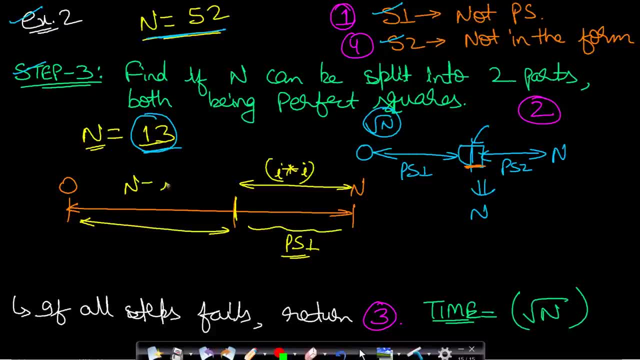 so how will you do this? so this value will be nothing but n minus i into i. so you will take the square root of this part and then you will check if square root of n minus i into i multiplied by the same value, which is nothing but the square root of n minus i into i. 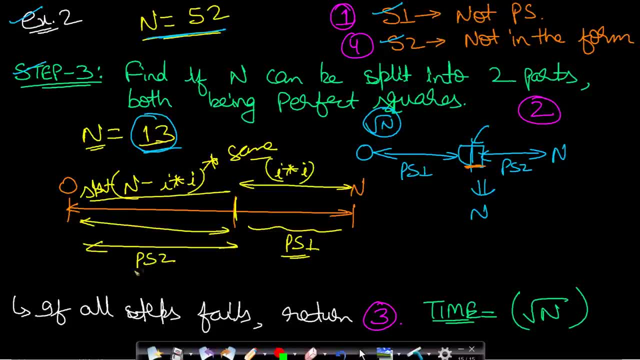 should be equal to this gap. okay, so then it will become a perfect square. and if it is a perfect square, then we have found a valid break point and we will simply return our answer to be 2, because this n can be formed by using two perfect square sums. so if we are not able to find any break, 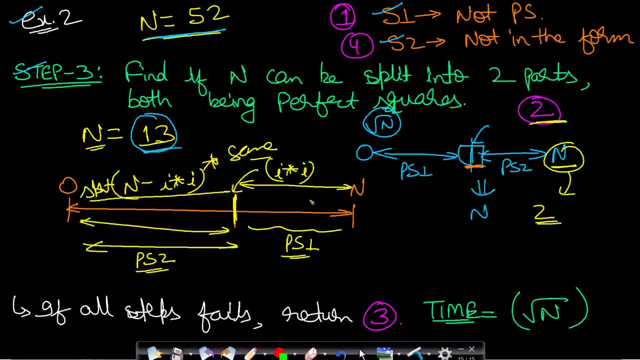 point which can divide a value n into two perfect square sums, then actually, this case for returning 2 is also gone. and now, since, according to lagrange's four square theorem, every natural number can be represented as a sum of four square sums. therefore, we have already 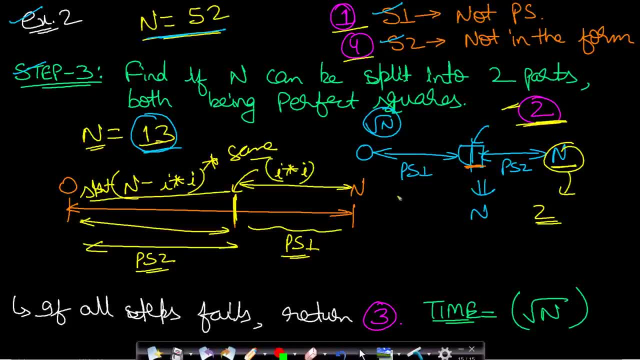 checked for case one, four and two, so our obvious answer will be three. so we will not do any checks for this three and we will simply return this three in step four. okay, so our total time complexity for this process is order of root n. so i hope you understood all the three processes. let us now look. 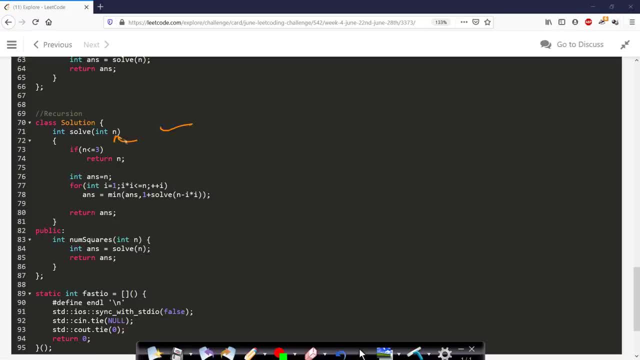 at the code. so this is the recursion code, where we are given n value and i have used simple recursion. okay, so this is our main function. actually, from here, i have called the recursion function and this is creating the breakpoints. so this is the first approach. let us now look at the second approach. 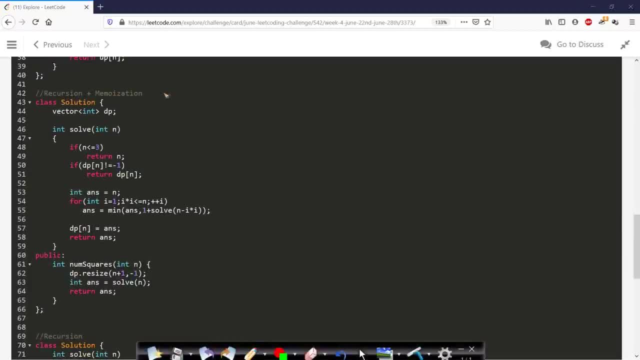 well, this second approach is based on recursion plus memoization, which is also dp, using a lookup table. so in this case i have used the same recursion code, but then this is only checking if the lookup table is also correct. so this is the first approach. let us now look at the second approach. 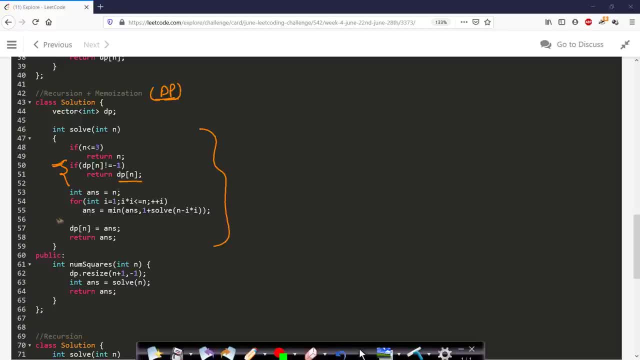 so this is the first approach. let us now look at the second approach. so this is the first approach. then we will simply return the value, otherwise we will calculate, and after calculating we will populate our dp table. so in this way we can use memoization. now let us look at the next. 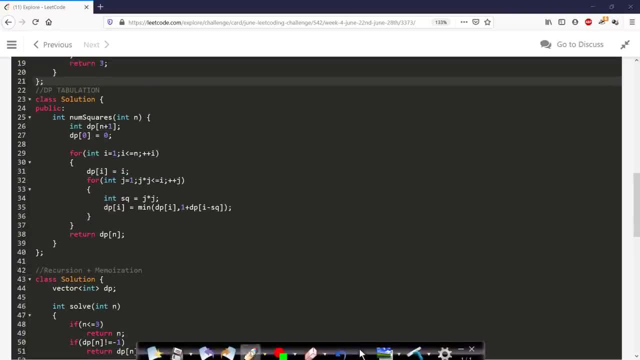 method. well, the next method is based on dp tabulation. so this is also very simple where we are given this n value and i have made a single dimensional table, okay, and in this case i have just filled dp at 0. in the theory part i have shown that i filled 0, 1, 2, 3, so you can follow that. 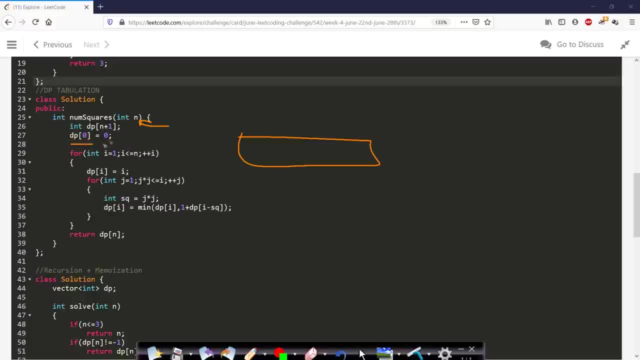 or you can do like this: just fill dp at 0 equals 0, and then again i have followed the same process. i have processed each and every number, from 1 to n, and for each number i have assigned the current cell with the value i, because this is the maximum number of split. so if you are at this number 2, 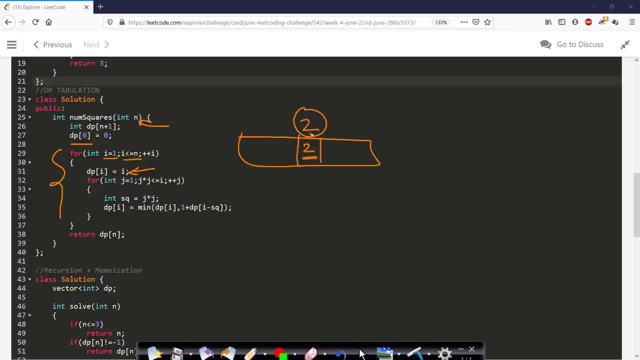 then initially i was showing that it will be 2. 2 will be filled, because we can always break a number into chunks of 1 square. now, since this is filled, this is the maximum, or divisions after that. we will try to minimize this. so we will try to create chunks. 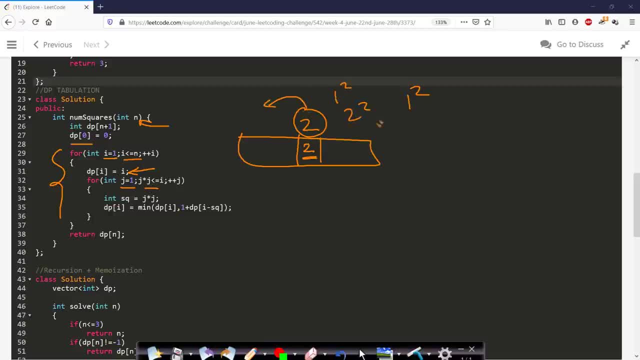 so we can create breakpoints at 1 square, 2 square, 3 square and so on, and whenever we make a breakpoint then actually we will be comparing 1 plus dp at i minus square. that is the breakpoint and the current value which is already stored. so this i have already. 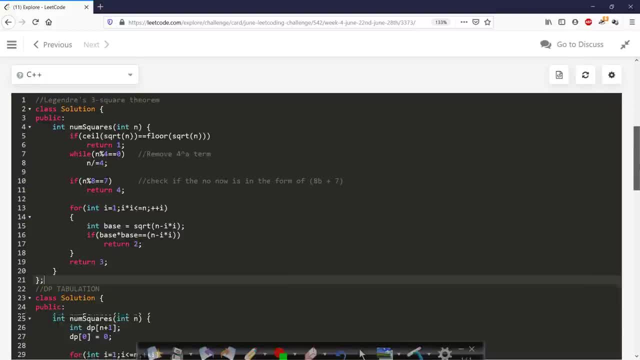 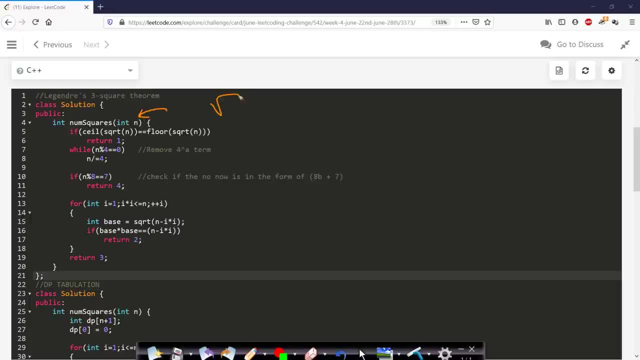 explained in the theory. now let us look at the next method. this is the last method, which is by groups of ع, 24 Light J is here, so, ah, flip the vector box to the center, OR, if you will hiring i as false, then start the rotate to somewhere here. let us consider this as the target 2 and our junior. 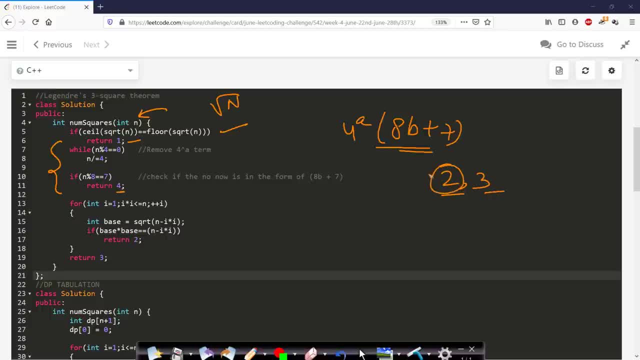 dear viewers, you will learn a few basic exercises of Xiao posture questions, including the vertical rotation chart and recovery method. we also will gather another one in future. so that is the problem which we will solve: to solve this problem in in the next tape and time. so in this case, 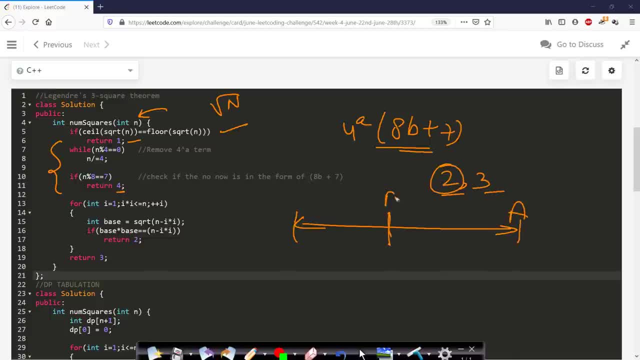 can be divided into two parts, making a breakpoint at some position such that this one is also a perfect square and this one is also a perfect square, then we can return two. okay, so we are creating the breakpoints at a split point of perfect square. so in this case, you can see that. 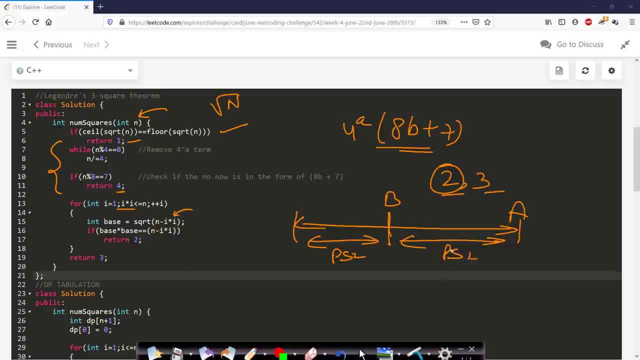 we are splitting at perfect square values n minus i square. so this one, uh, this right side one, is already ensured that this is a perfect square, since the breakpoint size is of perfect square, starting from a. okay, so now we just need to check this part if it is a perfect square, if this second